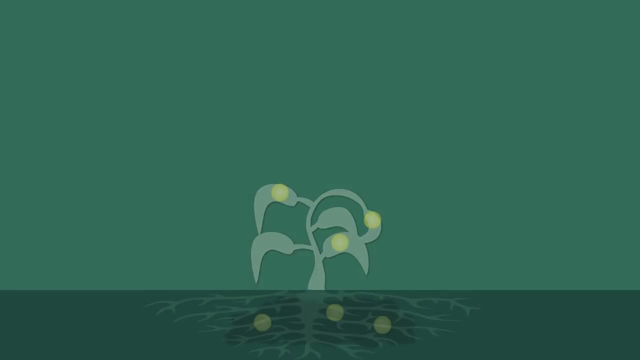 plants die and eventually form coal and oil. over millions of years. these sulphur atoms remain bonded to the carbon atoms. The sulphur content of coal and oil are then added to the carbon atoms. An oil is usually between one and four percent by weight. What do you think is produced when? 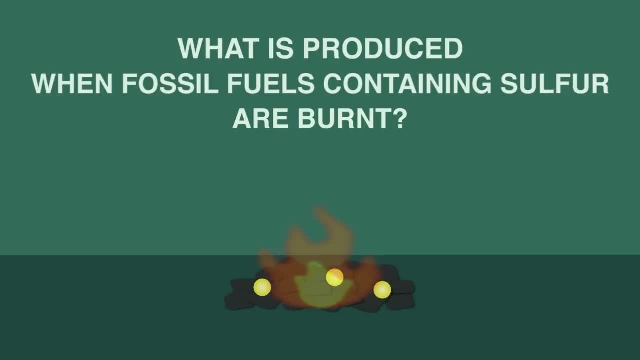 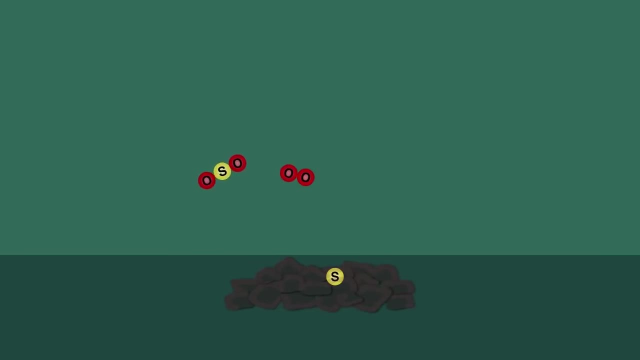 fossil fuels containing sulphur are burnt. Pause the video whilst you think. When the coal is burnt, the sulphur and the carbon atoms join with oxygen from the air and are released into the atmosphere as carbon dioxide and sulphur dioxide In the presence of sunlight. 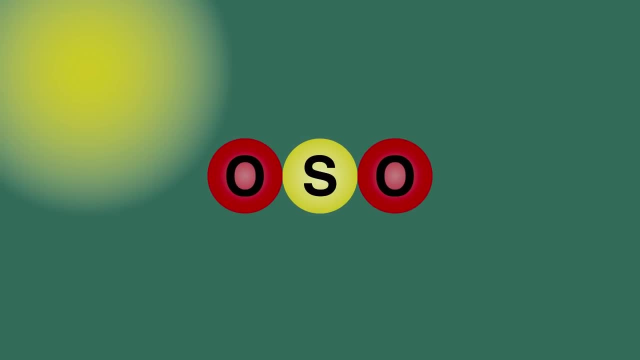 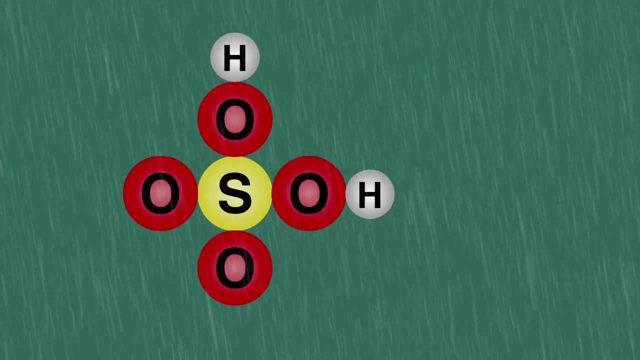 a chemical reaction will take place where sulphur dioxide reacts with more oxygen to form sulphur trioxide. This dissolves in the rainwater, forming sulphuric acid. Let's now consider how nitric acid gets into the rain In the high-temperature conditions in the 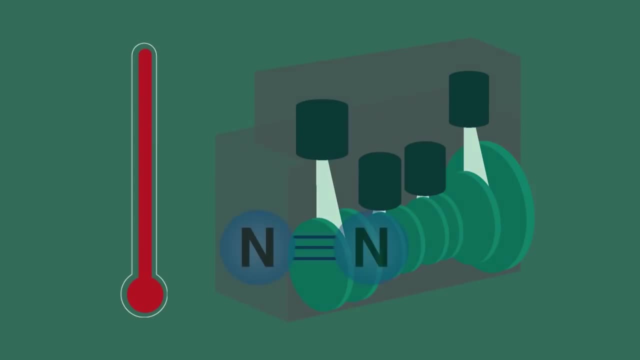 cylinders of our motor vehicles. a small amount of nitrogen and oxygen from the air can react. Remember that air taken in to combust the fuel is nearly 80 percent nitrogen, so exhaust gases from vehicles contain small but significant amounts of nitrogen oxides. Once the oxides of 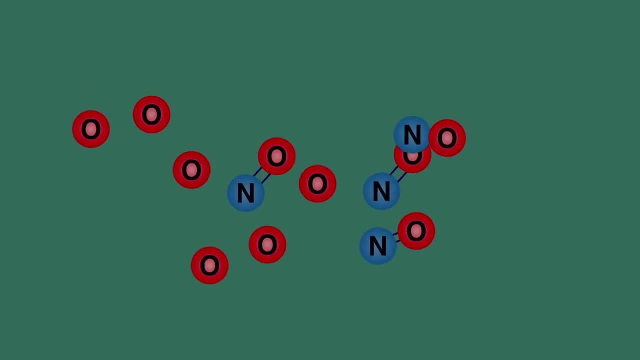 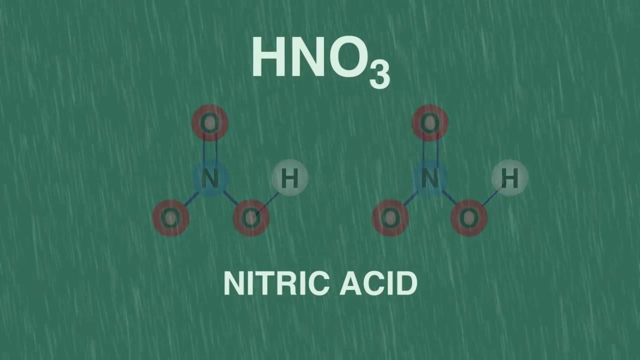 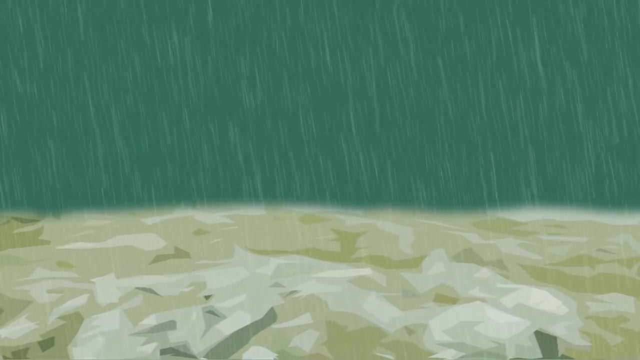 nitrogen are in the air. they react with more oxygen, just like we saw with sulphur dioxide, and dissolve in the rainwater to form nitric acid. If the rain falls on limestone soils, which are alkaline, the acidity may be neutralized. However, if the rain lands on neutral or acid soils, 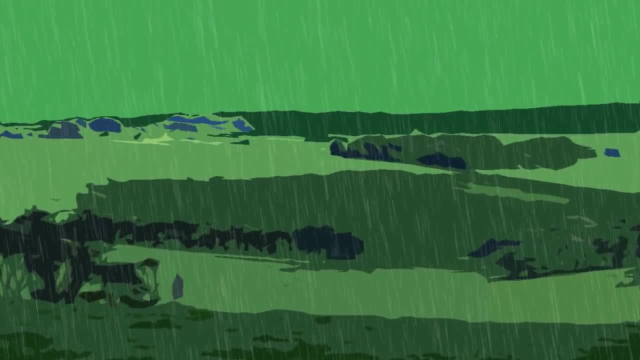 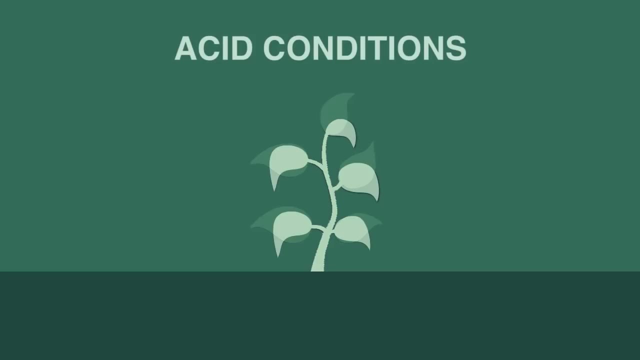 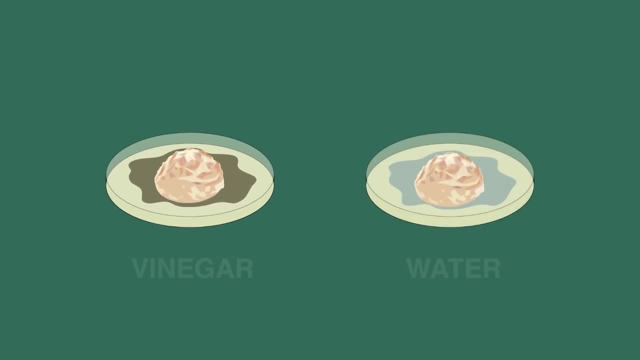 or on vegetation, then it can cause damage. So why is this acidity harmful to living things? Well, living things don't grow well in acid conditions, and it's easy to demonstrate this: Soak a slice of bread in vinegar and another in pure water. leave them open for a little while and then leave them covered. 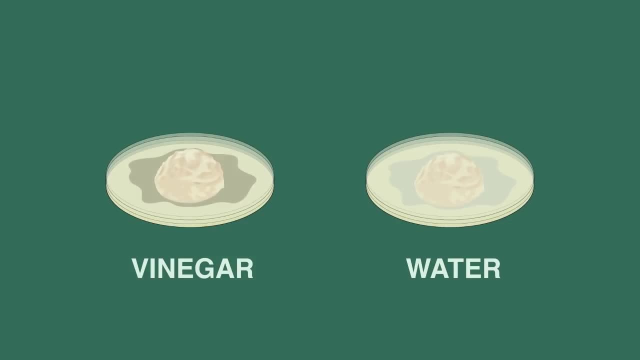 for a week, You will find that the bread soaked in vinegar has not gone moldy, whereas the other bread has. In fact, we use vinegar to preserve food in a process called pickling. This is the case because certain enzymes, which are vital for growth, are unable to function.